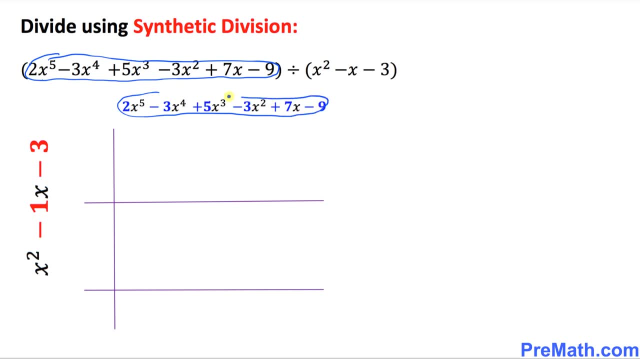 I just wrote it down on the top of this chart And as far as this divisor is concerned, I put down divisor on this one left hand side. Make sure it should be on this side. And this next step is really crucial. So you see, these coefficients of this dividend to. I just put it down by itself over here. The next coefficient of 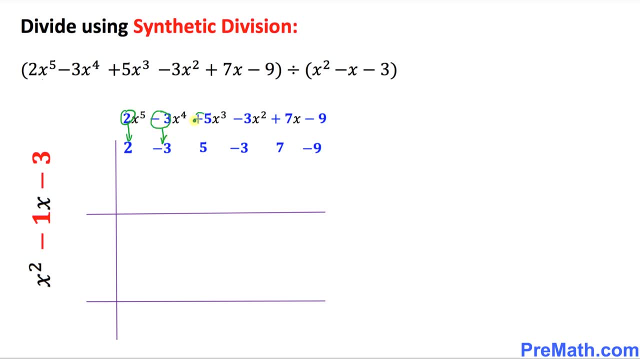 X power: 4 moves down to over here. Likewise, this is positive 5.. Negative: 3 moves down over here. This is positive, 7. And this is negative 9.. Now let's focus on this polynomial on the left hand side. Look at this one First. I want you to focus on this part. 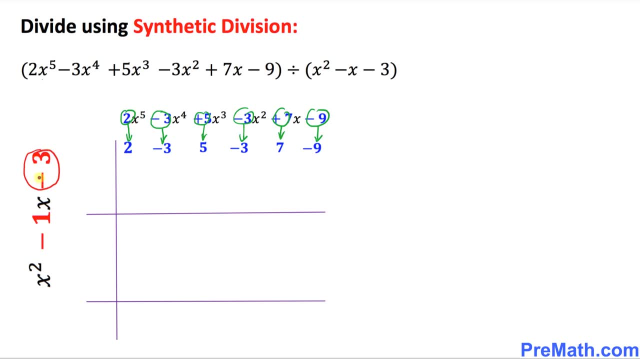 Constant part: Negative 3.. The opposite sign of negative 3 is positive 3.. So positive 3 is going to show up in this box on the top. And as far as this middle number, negative 1, is concerned, we do the same thing. The opposite sign of negative 1 is positive 1.. And it is going to show up in this second box. 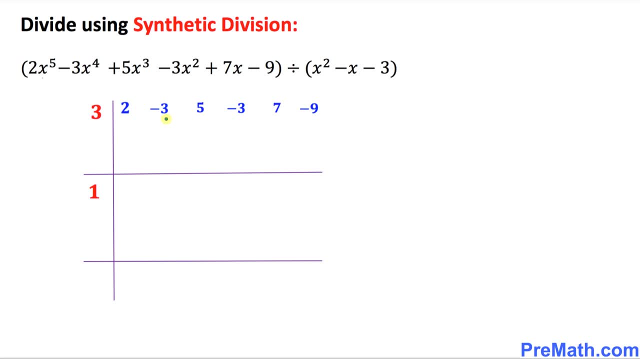 And here is the final product. We put down all these constant numbers, The coefficients, on this one horizontal way and on the vertical way, before we get started with our synthetic division. And here is the very first step. You see this 2 over here, The first number. I want you to drag it down all the way over here at the bottom. 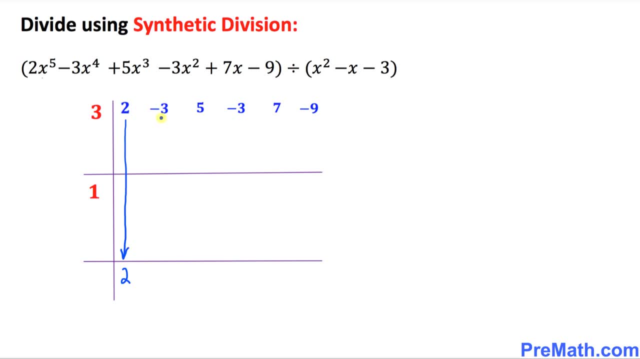 So 2 shows up over here. far as this next number, negative 3, is concerned, drag it down to right here in this box. so far, so good. so the next step is we are going to multiply this one. I want you to multiply this 1 times 2, diagonal way, 1 times. when you do this, 1 times 2 is 2, so this 2 is going to show. 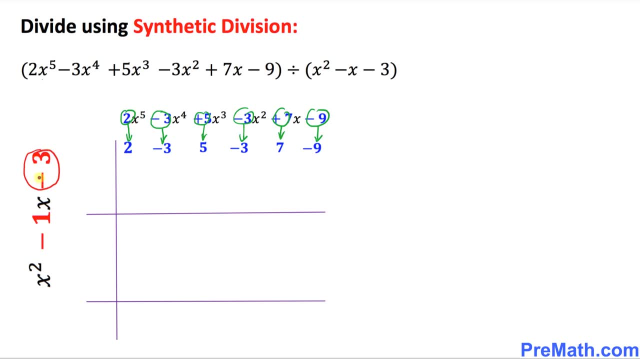 Constant part: Negative 3.. The opposite sign of negative 3 is positive 3.. So positive 3 is going to show up in this box on the top. And as far as this middle number, negative 1, is concerned, we do the same thing. The opposite sign of negative 1 is positive 1.. And it is going to show up in this second box. 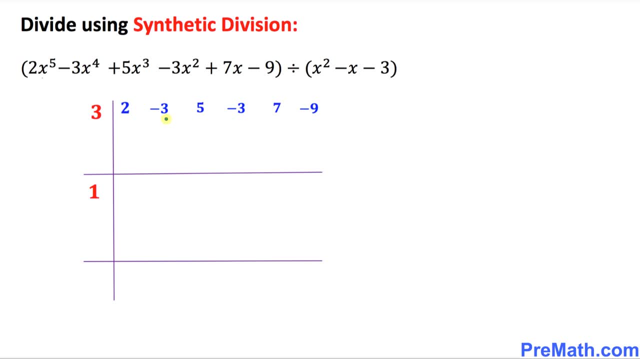 And here is the final product. We put down all these constant numbers, the coefficients, on this one horizontal way and on the vertical way, before we get started with our synthetic division. And here is the very first step. You see this 2 over here, The first number. I want you to drag it down all the way over here at the bottom. So 2 shows up over here. As far as this number goes down, 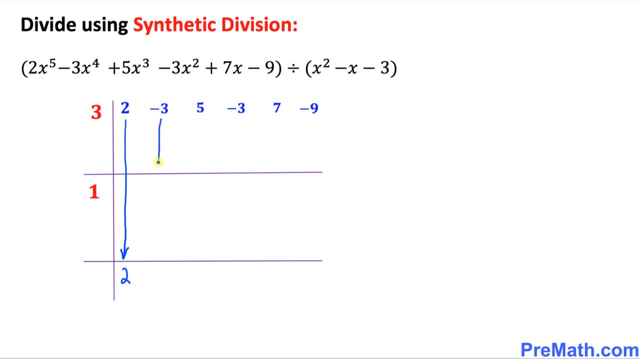 As far as this next number, negative 3, is concerned, drag it down to right here in this box. So far, so good. So the next step is we are going to multiply this one. I want you to multiply this 1 times 2.. Diagonal way. 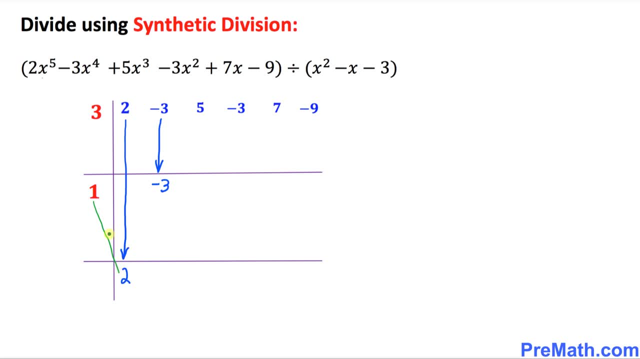 1 times. when you do this, 1 times 2 is 2.. So this 2 is going to show up Right here, 1 times 2.. So it's going to sense you. This one is in this middle box, So it has to show up this thing. Likewise, this 3 is also going to get multiplied with this 2.. 3 times 2 is 6.. So 6 is going to show up right up here. So far, so good. So let's add these numbers now. 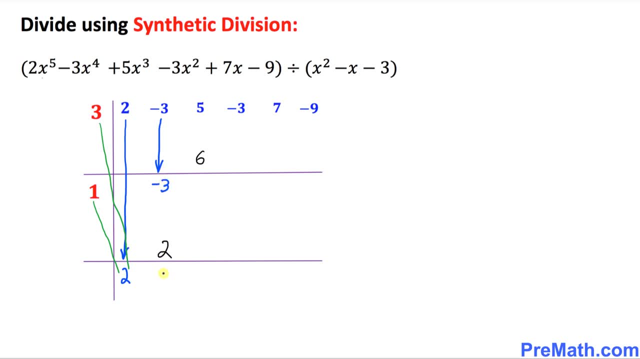 Okay, over here, Negative 3 plus 2 is going to be negative 1.. Likewise, 5 plus 6 is going to be 11.. All right, We're going to do the next step. We're going to repeat the same process all over again. Let's multiply 1 with this next number: negative 1.. 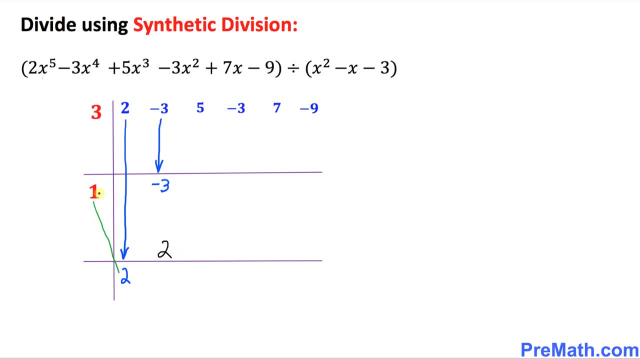 up right here: 1 times 2, so it's going to sense you. this one is in this middle box, so it has to show up this thing. likewise, this 3 is also going to get multiply with this. 2 3 times 2 is 6, so 6. 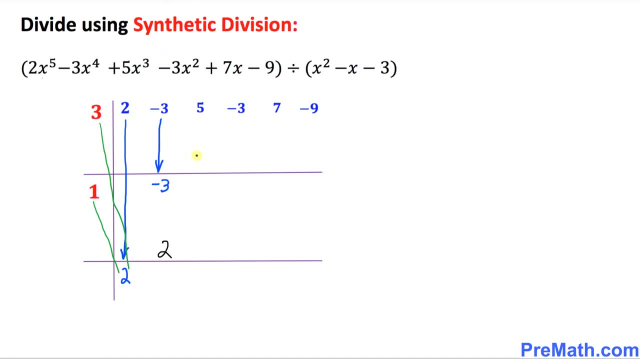 is going to show up right up here. so far, so good. so let's add these numbers here now. okay, over here, negative 3 plus 2 is going to be negative 1. likewise, 5 plus 6 is going to be 11. all right, we're gonna do the next step. we're gonna repeat the same process all over again. let's. 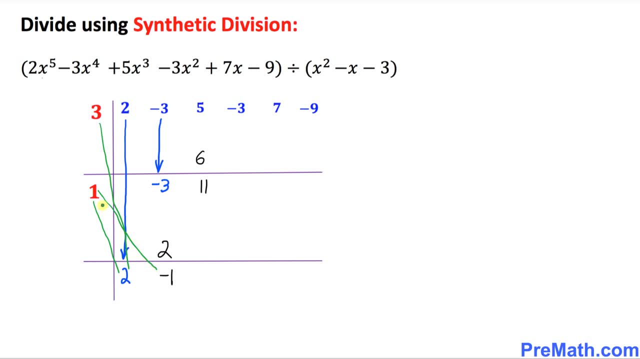 multiply 1 with this next number: negative 1. 1 times negative 1 is going to be negative 1. and likewise, this 3 is gonna get multiplied by this negative 1. this 3 times negative 1 is going to be negative 3. it's going to show: 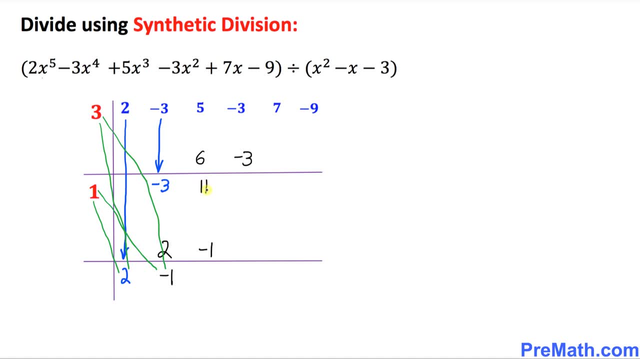 up over here. let's add these numbers again: 11 and minus 1 is going to make 10, right up here. and negative three. and negative three makes negative 6.. Let's start this process again. multiply this 1 with this 10.. one times 10 makes 2.. You'll see: Give 4 Mid 8な Types перевод. 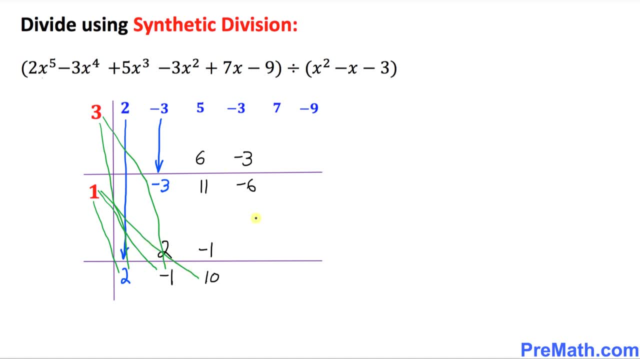 1 times 10 is going to be positive 10 right up here. Likewise, I'm going to multiply this 3 times 10 right now. 3 times 10 is 30. So 30 is going to show up on the top. 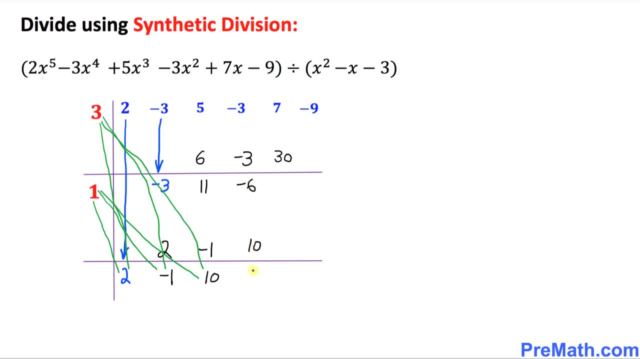 Let's add these: one So negative, 6 and 10 is going to make 4 at the bottom, And this one, 7 and 30, becomes 37. So far, so good. Now, finally, we're going to do one more time: This 1, just go ahead and multiply with 4.. 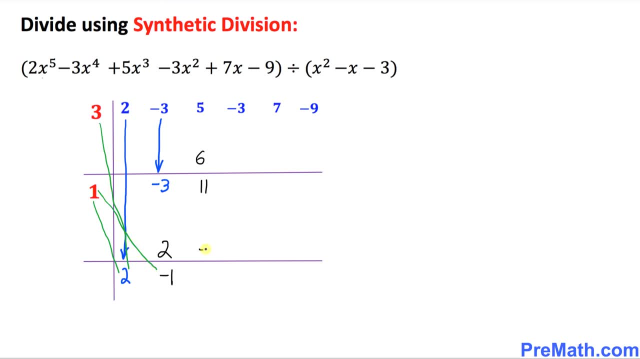 1 times negative, 1 is going to be negative 1.. And likewise, this 3 is going to get multiplied By this negative 1.. This 3 times negative 1 is going to be negative 3.. It's going to show up over here. 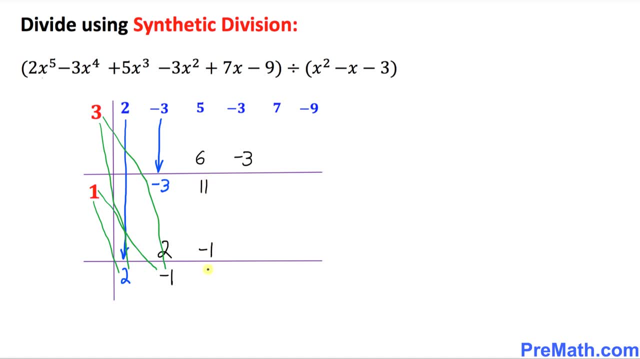 Let's add these numbers again: 11 and minus 1 is going to make 10, right up here And here negative 3, and negative 3 makes negative 6.. Let's start this process again. Multiply this 1 with this 10.. 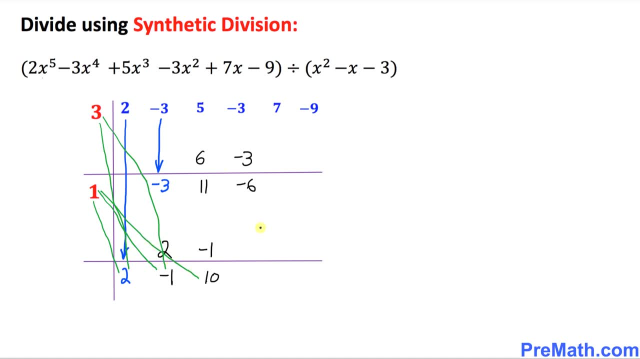 1 times 10 is going to be negative. 1. to be positive: 10 right up here. likewise, i'm going to multiply this 3 times 10. right now, 3 times 10 is 30, so 30 is going to show up on the top. let's add these one, so negative: 6 and 10 is. 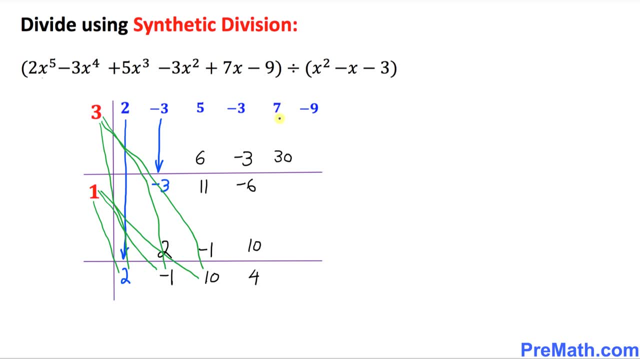 going to make 4 at the bottom, and this one 7, and 30 becomes 37. so far, so good. now, finally, we're going to do one more time. this one: just go ahead and multiply with 4. 1 times 4 is going to be 4. 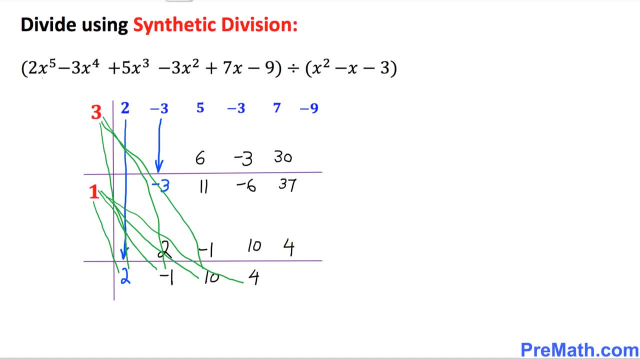 right up here, and likewise this 3 is going to get multiply by 4. 3 times 4 is going to be 12 right up here. so that is now we're going to add these 37 plus 4 is going to be 41 right up here and negative 9. 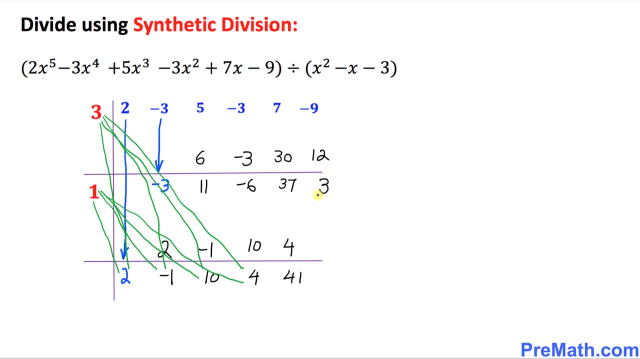 plus 12, and you added that's going to be 3. we are pretty much done. now the next is final step is i want you to bring down this positive 3 all the way at the over here bottom. so this 3 shows up right here. so this 3 is same as positive 3, by the way, isn't it? because this 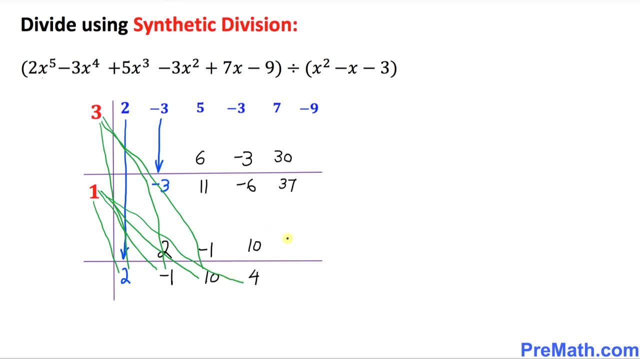 1 times 4 is going to be 4 right up here, And likewise, this 3 is going to get multiplied by 4.. 3 times 4 is going to be 12 right up here. So that is now. we're going to add these. 37 plus 4 is going to be 41 right up here, And negative 9 plus 12, and you added that. 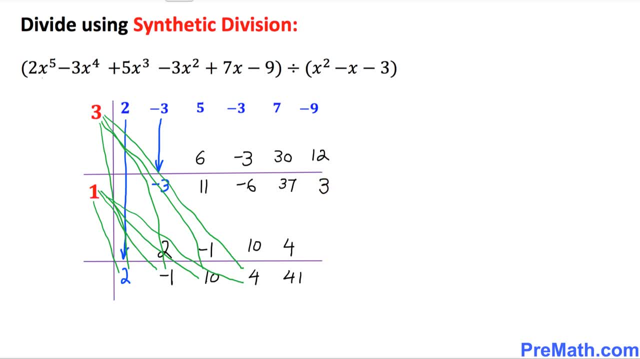 It's going to be 3.. We are pretty much done now. The next final step is: I want you to bring down this positive 3 all the way at the over here bottom. So this 3 shows up right here. So this 3 is same as positive 3, by the way, isn't it? Because this is what it is. 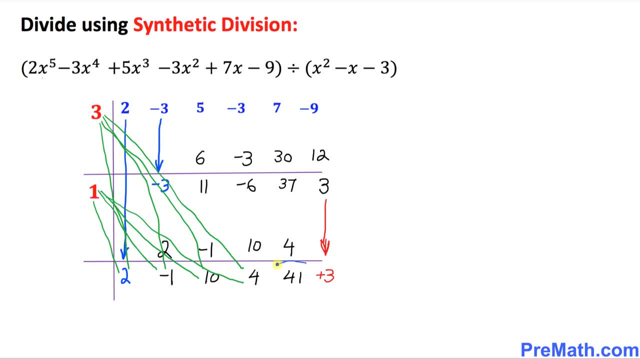 So now this whole part Is our remainder part And now, as far as you can see, this is the first number. 41 is going to be a with X, And this is the next number is without X, because this is like an X and this is a constant term. 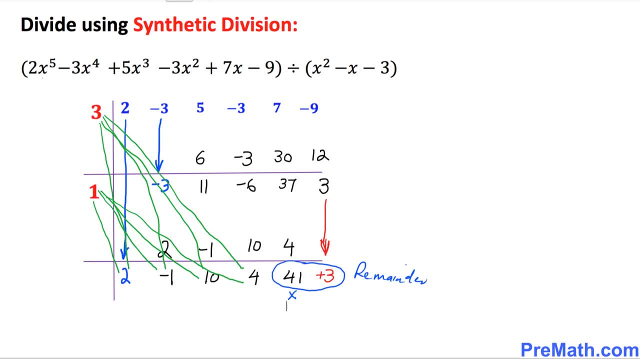 So that is going to be a simply is going to become 41 X, And then the constant term is plus 3.. So our remainder is 41 X plus 3.. Now let's look at this part, right now over here, This one, the one that I am going to circle, this one. 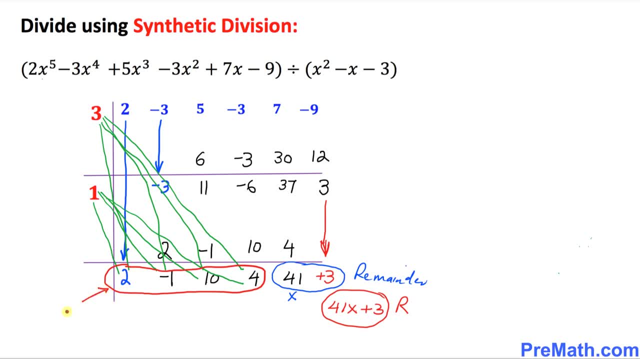 This part is called quotient, So let's focus on this one over here. This is: we see that we have a four term. always The first term is constant, The next one is 10, is going to be with X And this next one is going to be with X square. 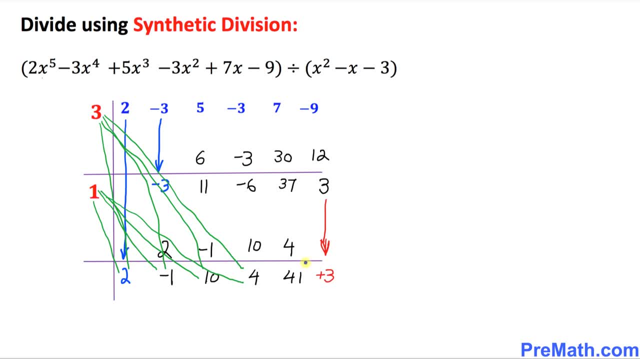 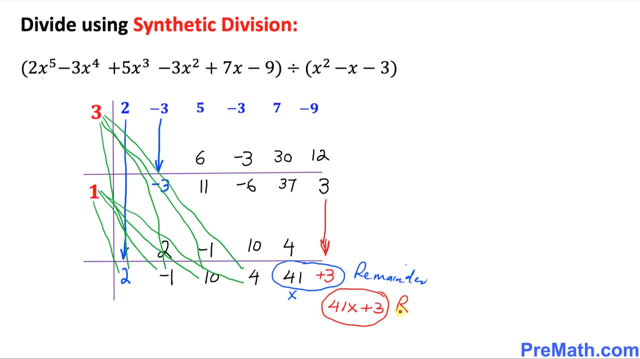 so our remainder is 41 X plus 3. now let's look at this part right now over here, this one, the one that I am going to circle, this one, this part is called quotient, so let's focus on this one over here. this is: we see that we have a. 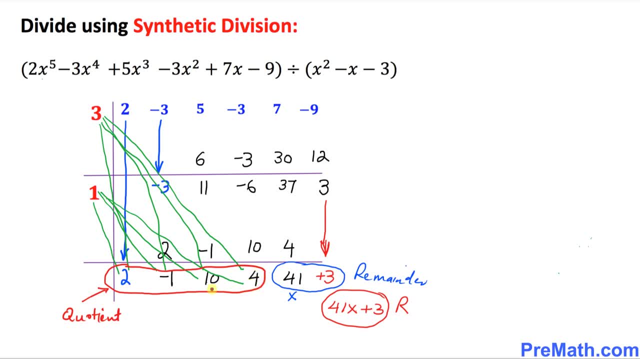 four term: always. the first term is constant, the next one is: 10 is going to be with X, and this next one is going to be with X square, and the next two is going to be X power 3, so this simply becomes a quotient, so let's focus on this one over here. this is we see that we have a. 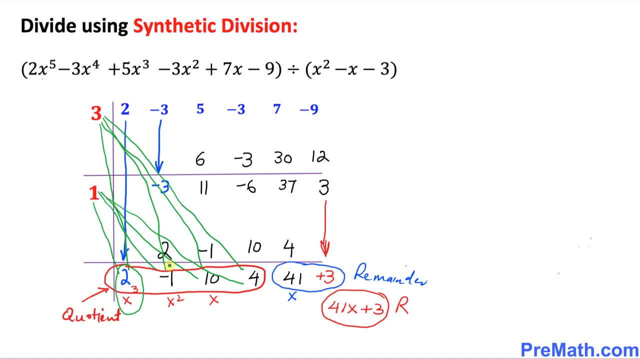 two X power 3 minus 1 X square, and this plus 10 X. this, if there's no sign, plus 10 X plus 4, so I can write this whole thing as 2 X power 3 minus 1 X square plus 10 X, and this become positive. 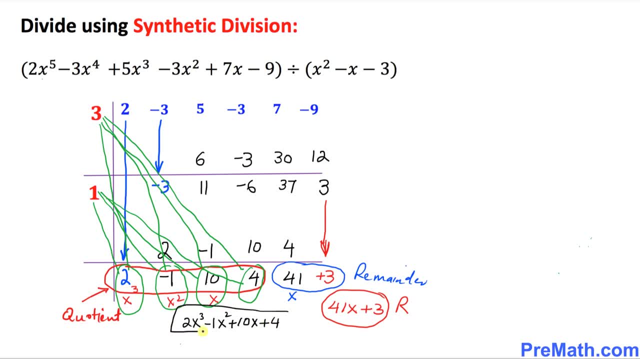 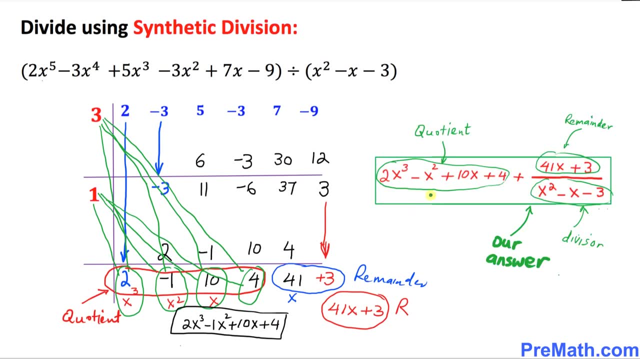 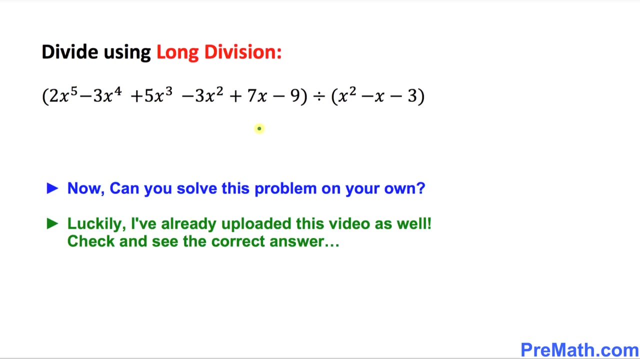 4 and this part is our quotient and this is our complete answer in this box. so, once again, this on the top part, this remainder, this the bottom one, is divisor and this one is our quotient. and here is your assignment. can you do the very same problems by using the long division? you can take your time. 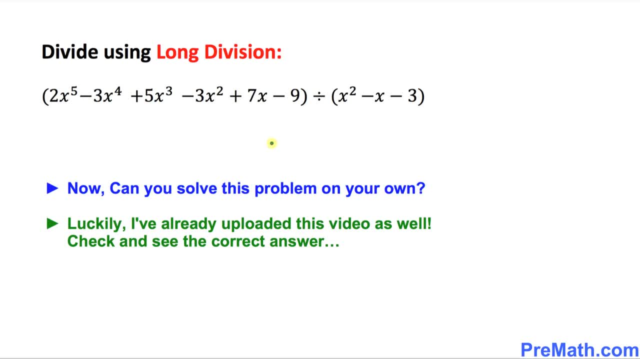 you can pause the video. luckily, I have already uploaded this video as well. please go ahead and check it out and see the correct answer. thanks for watching and please don't forget to subscribe to my channel for more exciting videos. bye. 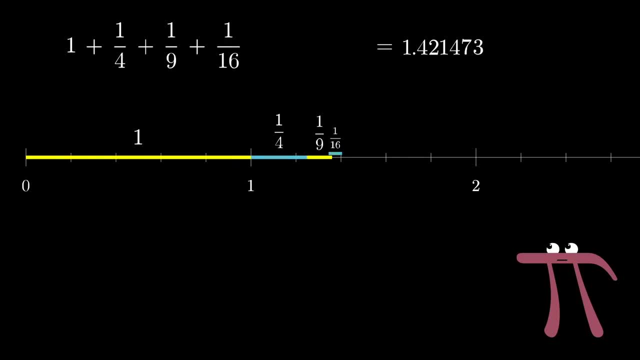 Take one plus a fourth plus one ninth plus one sixteenth and so on, where you're adding the inverses of the next square number. What does this sum approach as you keep adding on more and more terms? Now, this is a challenge that remained unsolved for 90 years after it was initially posed. 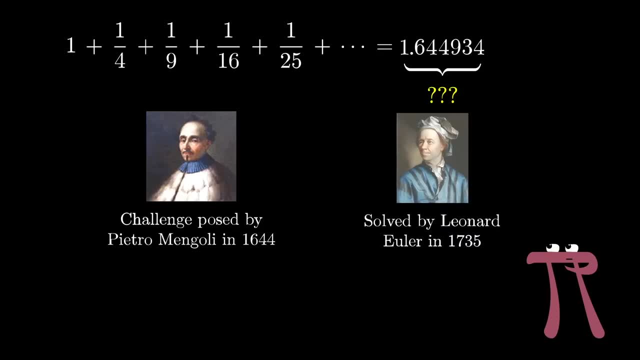 until finally it was Euler who found the answer, super surprisingly, to be pi squared divided by six. I mean, isn't that crazy? What is pi doing here, And why is it squared? We don't usually see it squared In honor of Euler, whose hometown was Basel. this infinite sum is often referred to. 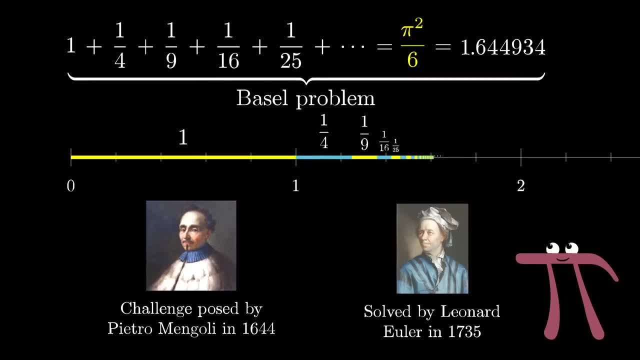 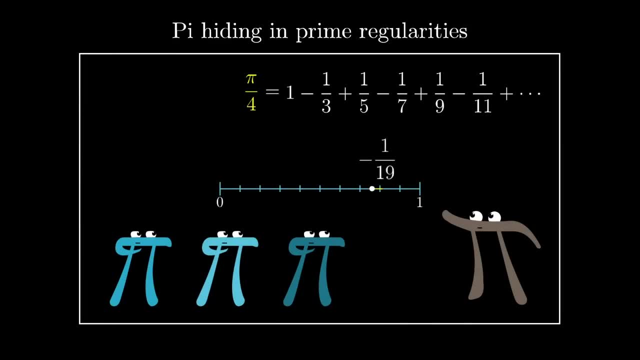 as the Basel problem, But the proof that I'd like to show you is very different from the one that Euler had. I've said in a previous video that whenever you see pi show up, there will be some connection to circles, And there are those who like to say that pi is not fundamentally about.